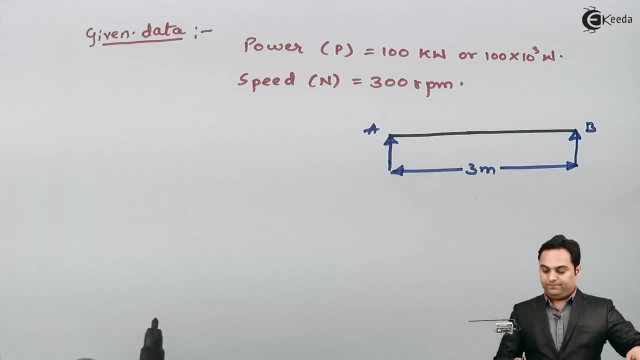 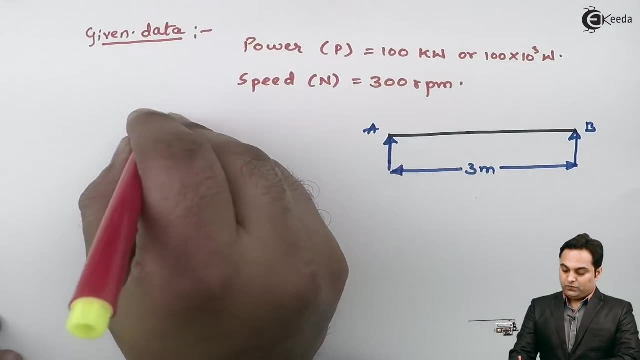 from the ends respectively. So here it is, given that this shaft, it carries 2 pulleys, each weighing 1500 newton, supported at a distance of 1 meter from the ends respectively, And their weight is given. that is weight of the pulley. 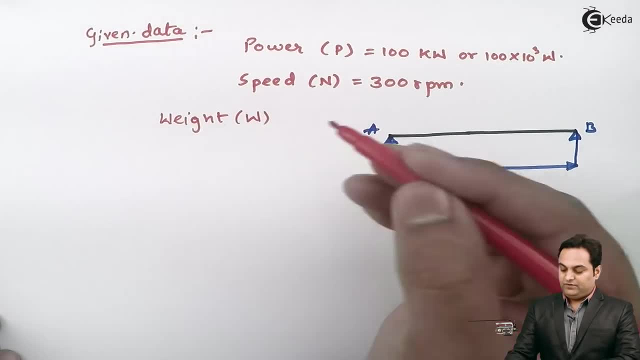 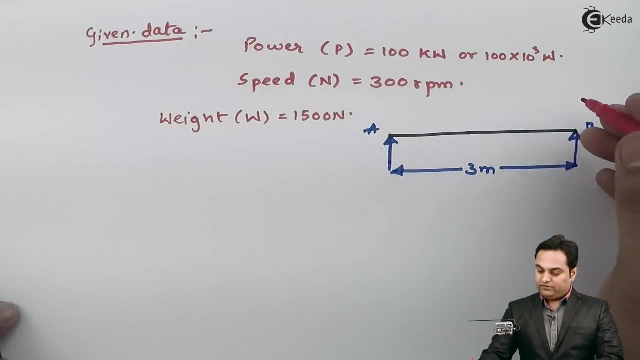 I will denote it by W, and that is equal to 1500 newton. So it means this shaft is going to carry 2 pulleys and they are 1 meter distance from each end. It means the shaft is going to carry 2 pulleys and they are 1 meter distance from each end. 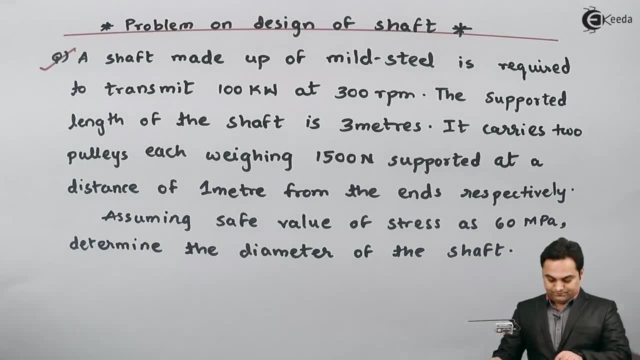 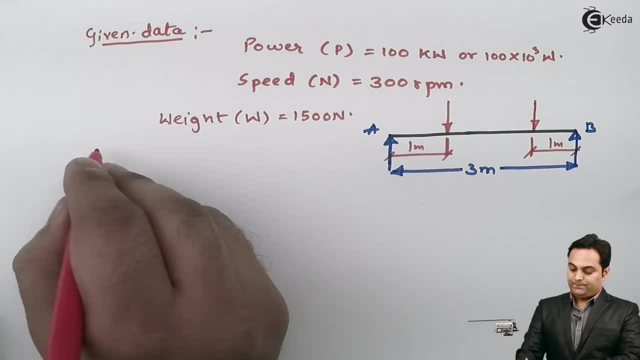 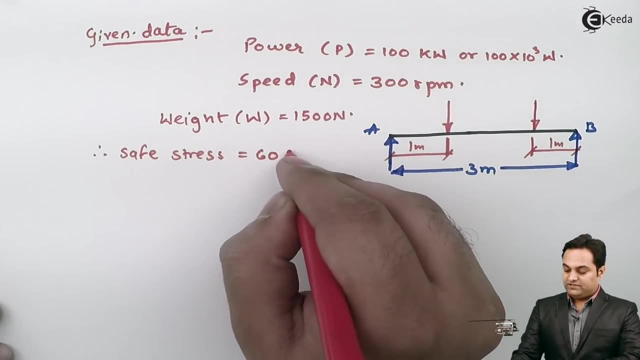 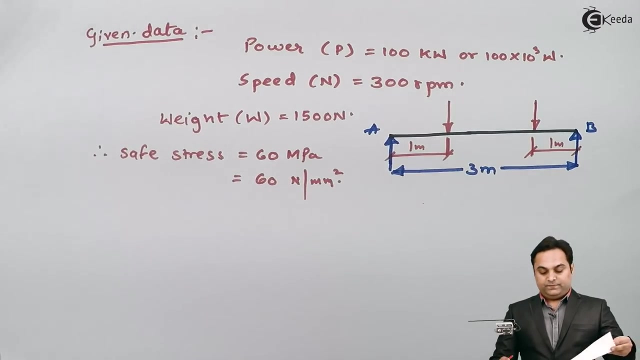 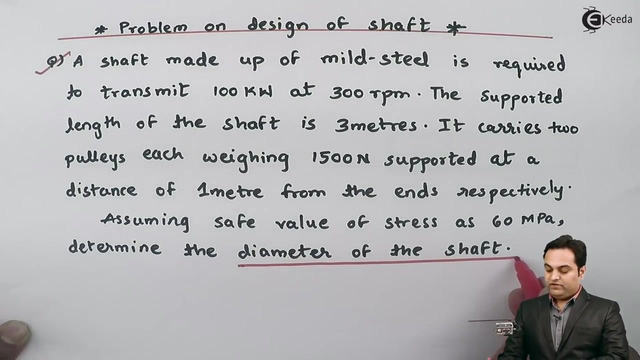 Next, assuming safe value of stress as 60 MPa. so this is the value of safe stress. given Safe stress is equal to 60 MPa, that is, 60 Newton per mm. square, Determine the diameter of the shaft. So this is the question for us. We have to find out how much would be. 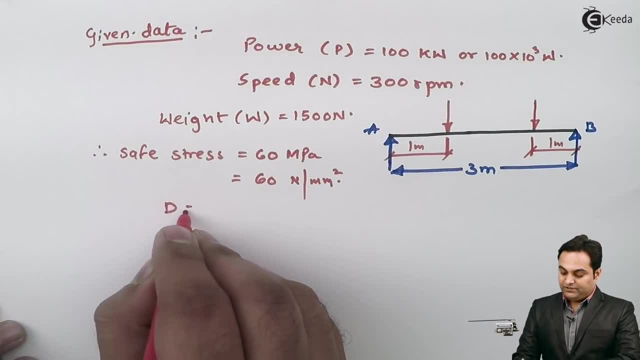 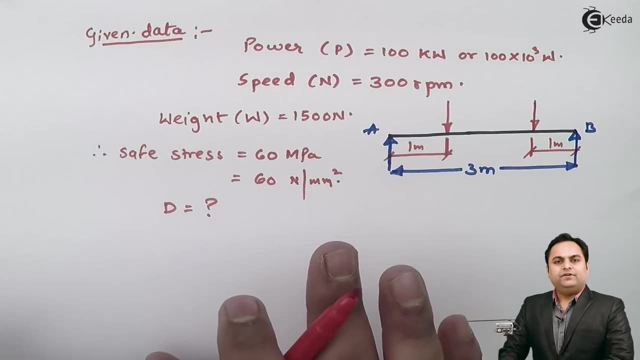 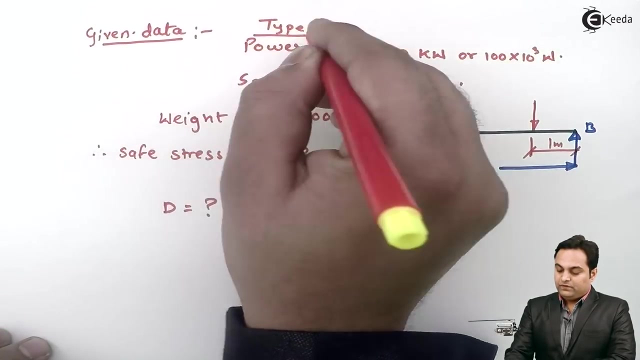 the diameter of the shaft So that I will denote it by capital D. Now, as we have seen in this problem, anywhere here it is not given that the shaft is hollow. So I can say that the type of shaft here it is a solid shaft. 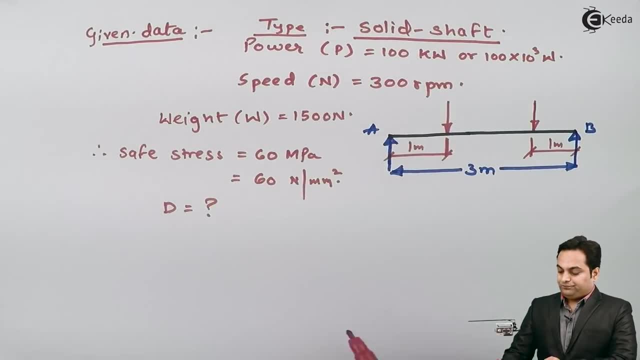 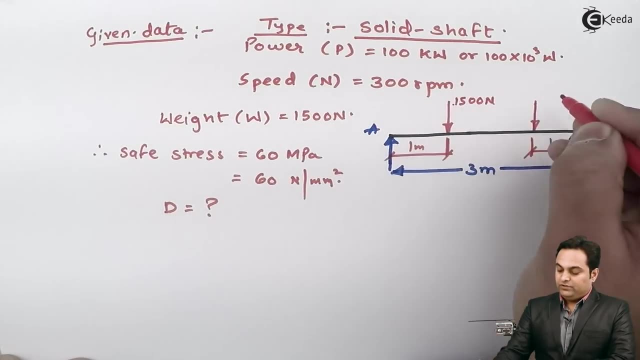 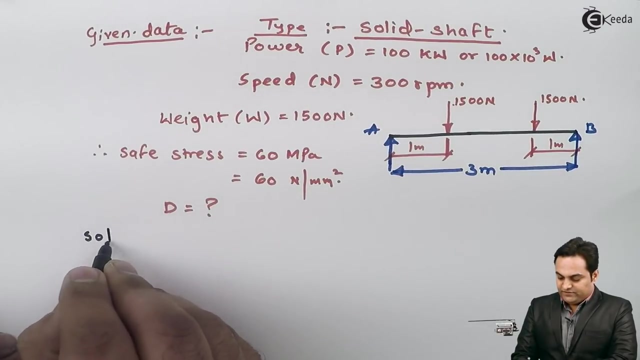 Okay, Now here, at both the ends, the pulley are there. Their weight is 1500 Newton on both the sides. So now this is the question with us. Let us try to get the solution for this problem. So in the solution part I will say that first of all I will explain this. 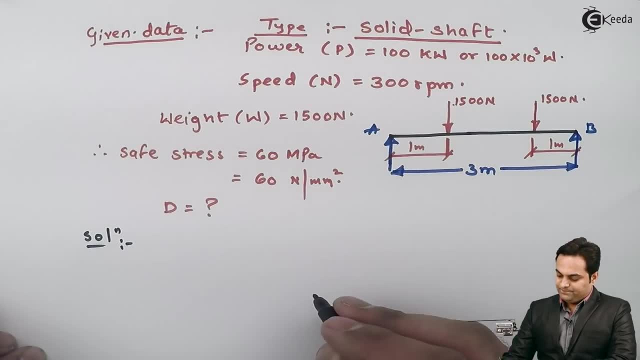 with a diagram more clear than this. Okay, Here I would be drawing a 3D diagram. This shaft: it carries two pulley and the weight of the pulley is same on both the sides. Their distances are also given in the problem, So 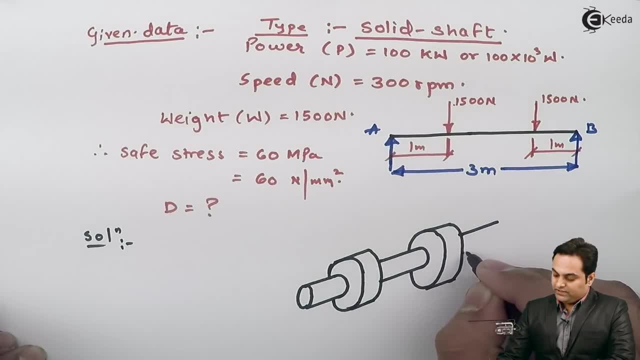 here. I have drawn this diagram. Now, as I have seen drawn in this diagram here, this is the shaft which is supported at two ends: Means at here: at this end it would be supported, and at this end, at the. 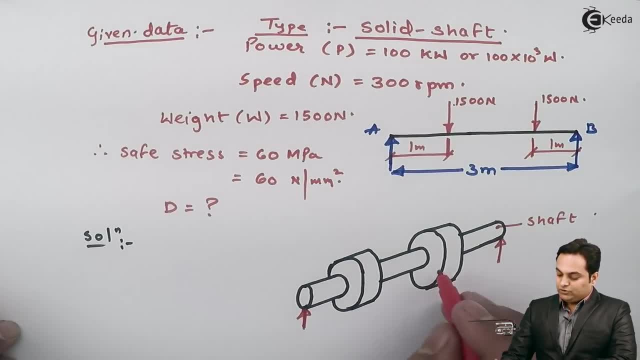 extreme ends This shaft. it carries two pulleys, as we can see here. These are two pulleys, These are two pulleys. Okay, I can say that this is also a pulley and here also we have a pulley. So what will? 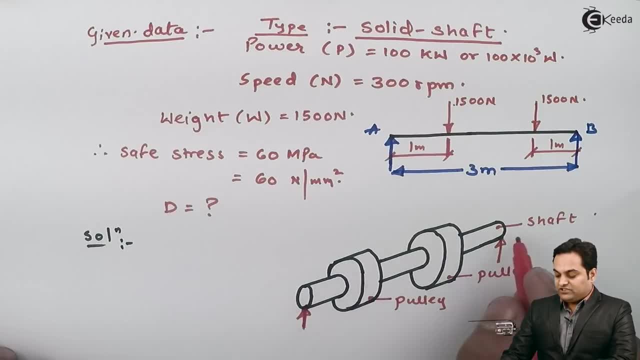 happen in this case is that when the shaft is supported between a length of three meter and then the weight of the pulley would be acting downward, So because of that, the shaft is subjected to bending. Because of the weight of the pulley, this shaft will. 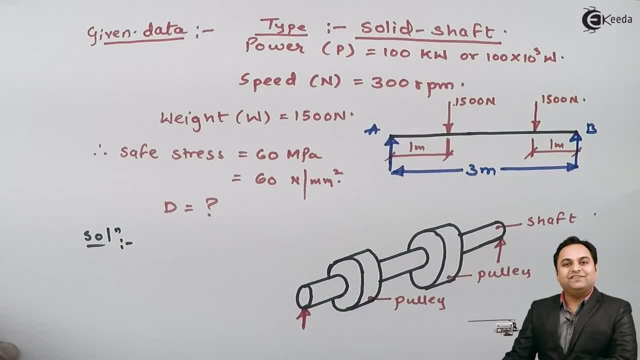 bend will try to pull the shaft in the downward direction, so there is bending of the shaft. at the same time, by the definition of shaft we know that it is a rotating machine element. so this shaft is constantly rotating and at the same time, when it is rotating, it is also subjected to bending because of the 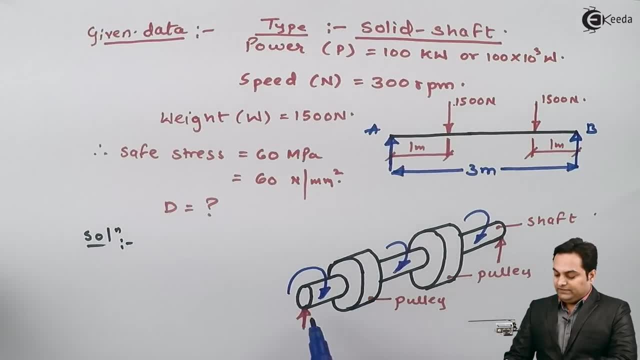 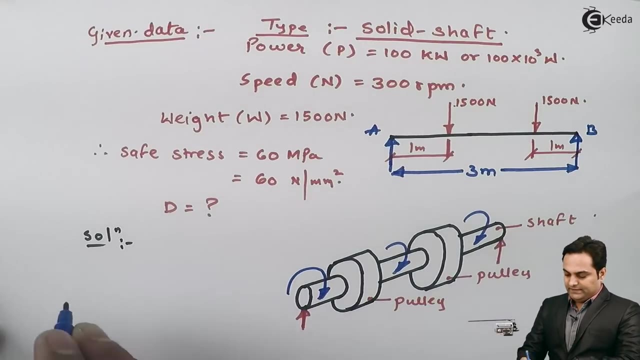 weight of the pulley on both the sides. so I can see that here this shaft is subjected to both, that is, it is subjected to twisting torsion because of the rotation and it is subjected to bending. that is, because of the weight of the pulley. so I can say that here the given shaft 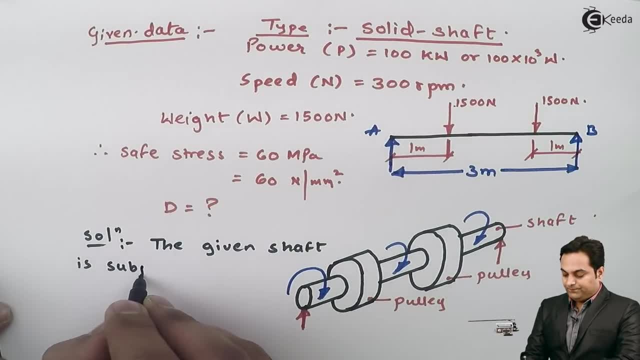 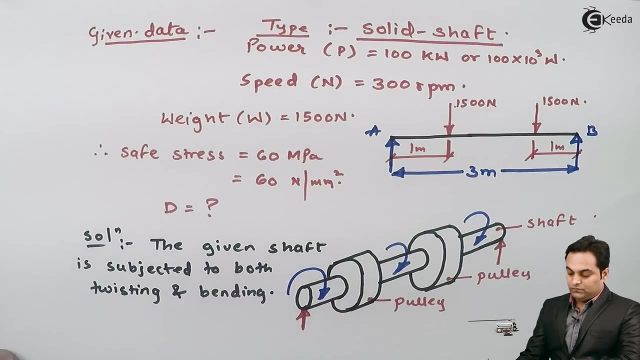 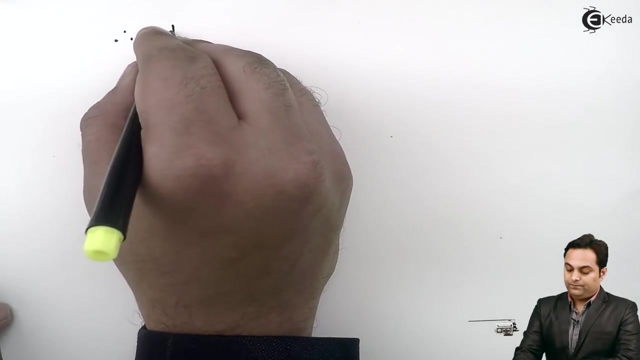 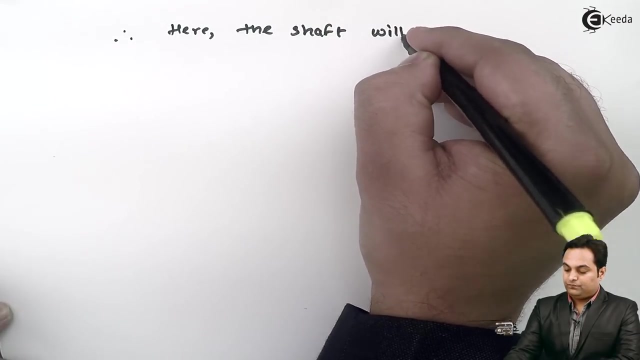 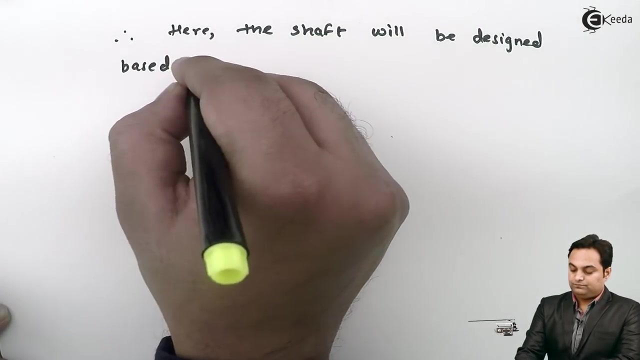 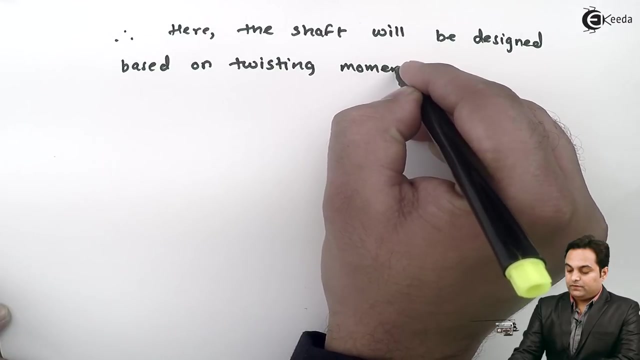 is subjected to to both twisting and bending. that is, the given shaft is since I will write down- since the given shaft is subjected to both twisting and bending. So therefore, here the shaft will be designed based on the twisting moment and the bending moment. Therefore, they will be designed according to the forward lat 96 cos theta on the curve. 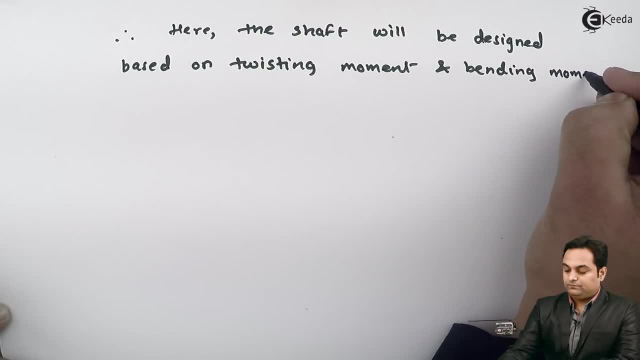 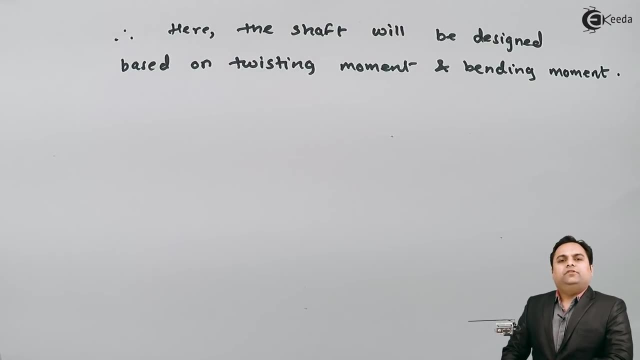 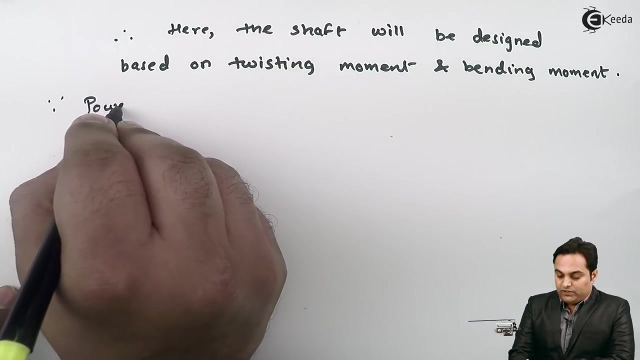 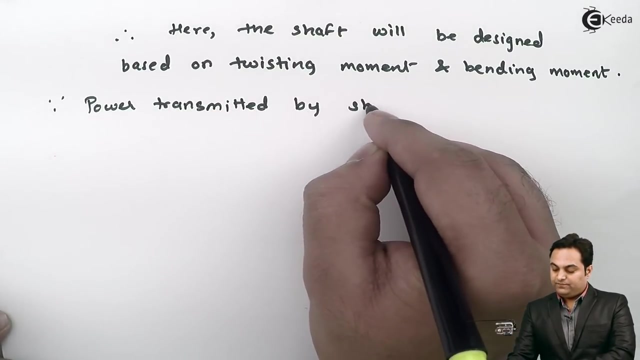 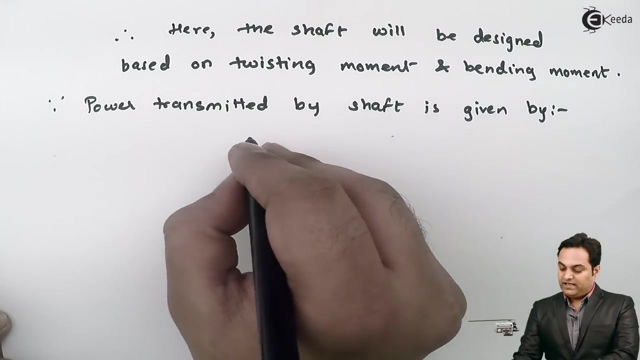 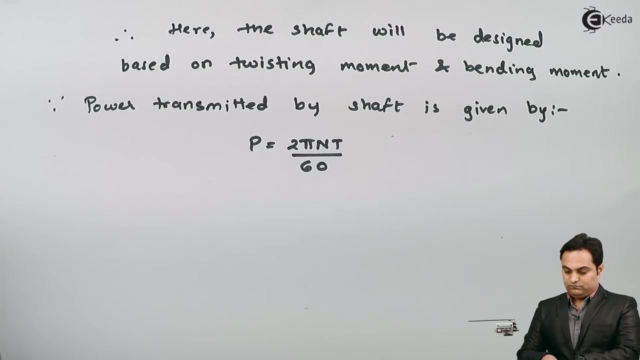 bending moment. so while designing this I will consider both twisting and bending now, since in this question they have given power, they have given rpm, so from that we can get the value of torque. so I will say that since power transmitted by shaft is given by power, as we know it is, P is equal to 2 pi NT upon 60. this is: 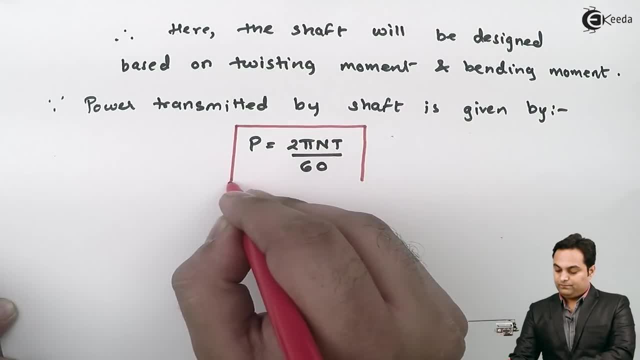 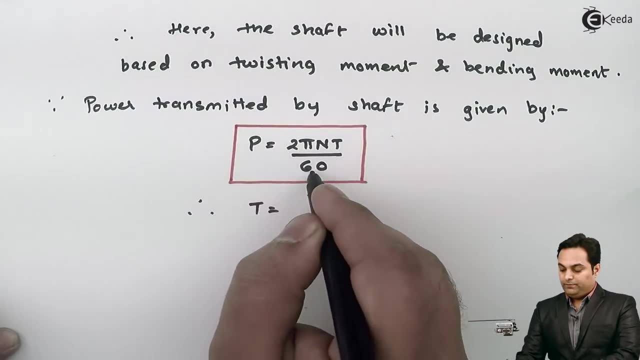 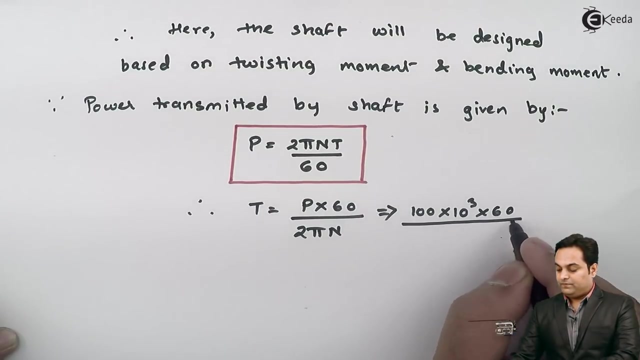 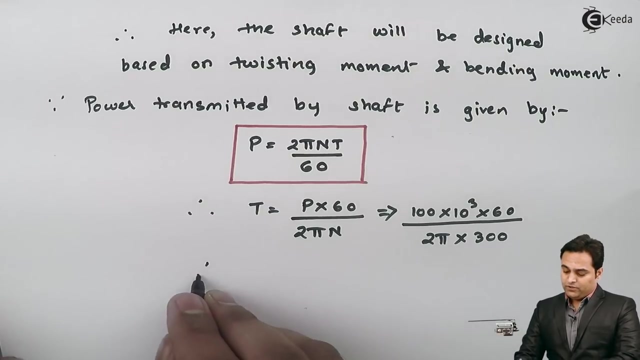 the formula of power. next, here I can say that therefore, torque T will be equal to P into 60 divided by 2 pi N. power it is given as 100 into 10 raise to 3 watts into 60, divided by 2 pi, into N is 300. that is the speed, 300 rpm. so from this I will get the value of. 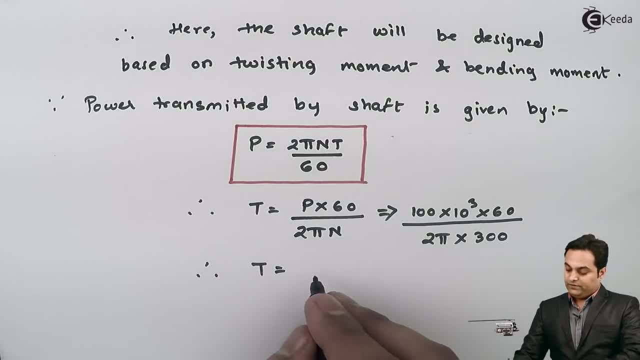 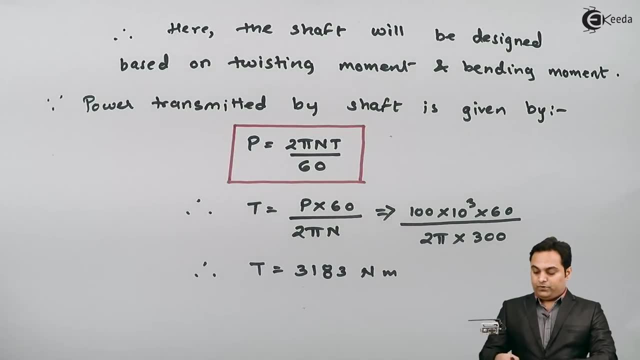 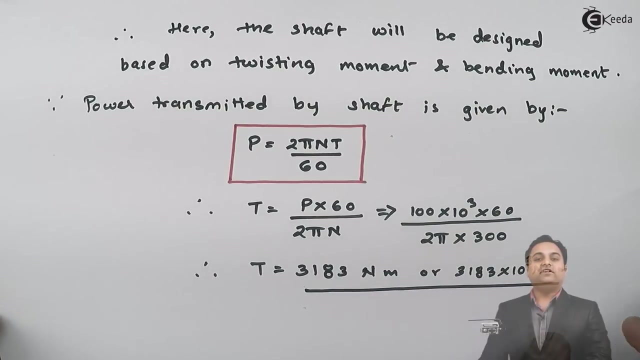 torque and my answer is it is 3183 Newton meter. now here we are getting torque in terms of Newton meter. I will also write it in terms of Newton mm. so it is 3183 into 10. raise to 3 Newton millimeters after getting the torque. 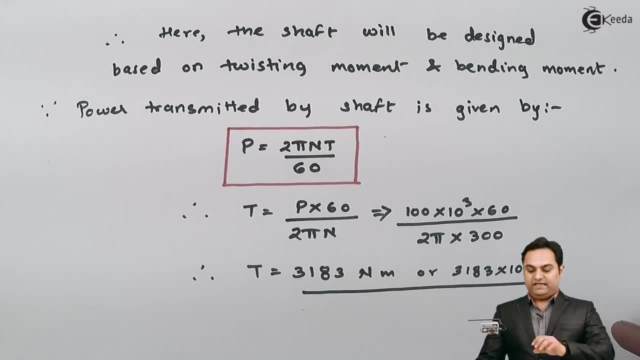 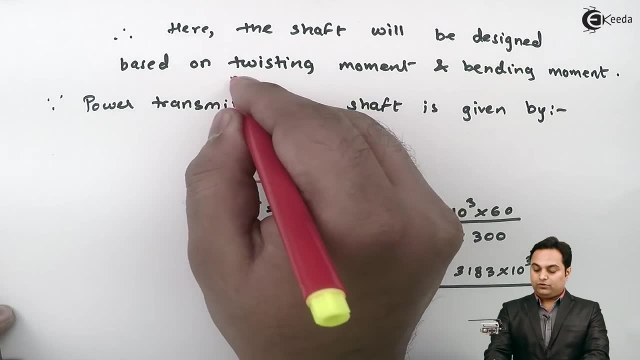 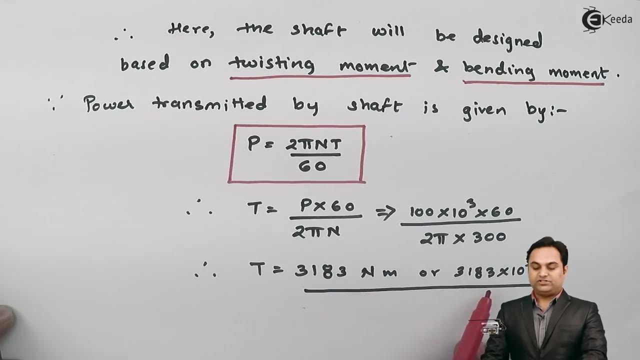 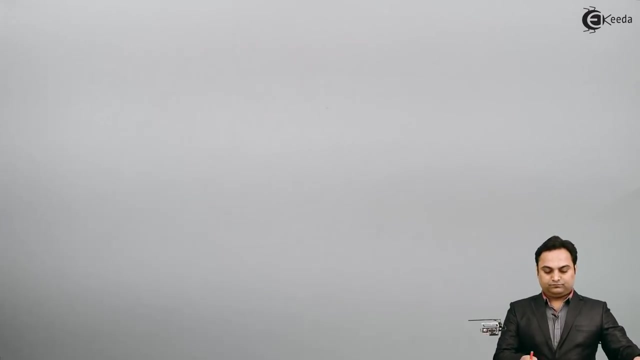 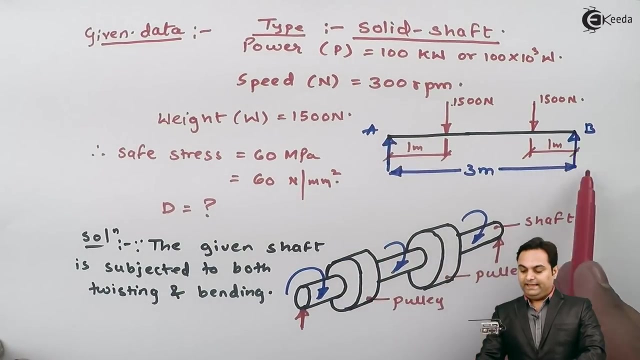 now I will go on to find the bending moment because, as I have told here that here we would be designing the shaft based on both twisting moment as well as bending moment. so twisting moment we have got just now. now I will calculate the bending moment and for that purpose I will say that, since the shaft is supported at a and b, 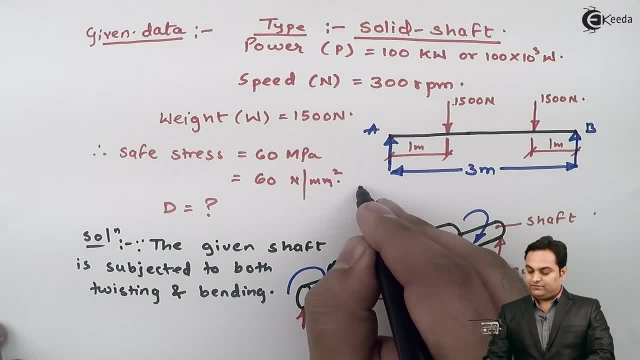 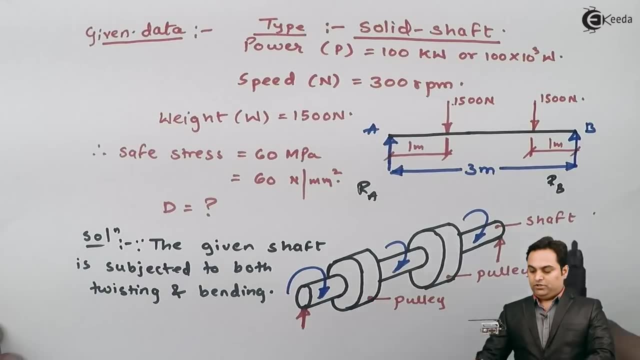 so here at a, we would be getting one reaction called as reactionity. here at b also, I would be getting one reaction, as we can see that I have given it to you and if I add this r A and this r b, now, how to get this r A and r b? see, it is very simple. as you look at this beam, it is exactly symmetrical. 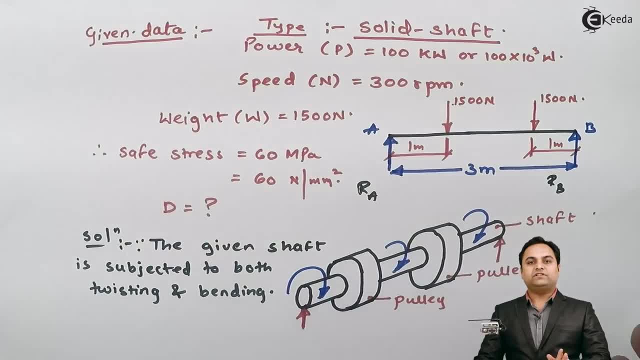 that is the loading, we can say the reactions, the loads. they are located at same distance from both the sides and even the load value are same. so if the total load, if I add this, that is 1500 and 1500, that gives me 3000 Newton. that 3000 Newton would be shared equally by both the supports. so it will be 3200 to 300 Newton. that gives me 3000 Newton. that 3000 Newton would be shared equally by both the supports. 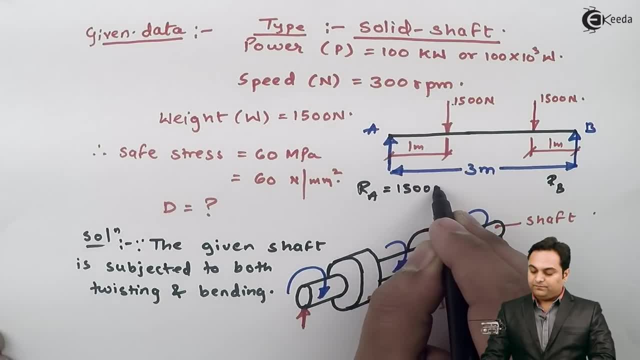 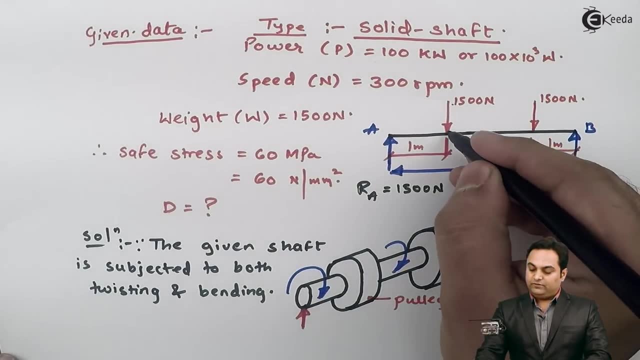 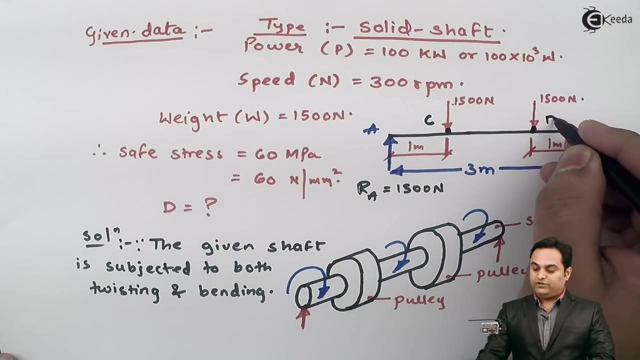 So at each support I am getting the reaction as 1500 Newton. So after getting R A and R B, now what I can do? I can calculate moment either at this, that is, I will say this is point C, or I can get the moment at this point, which is point D. 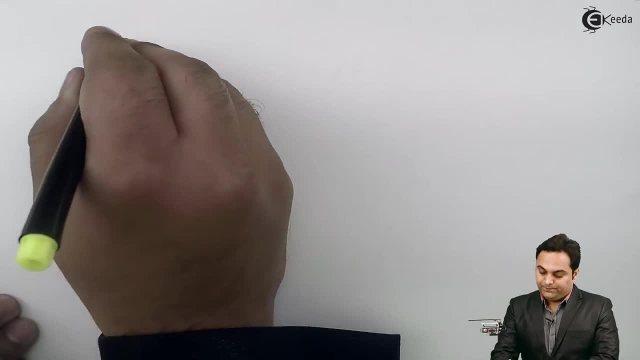 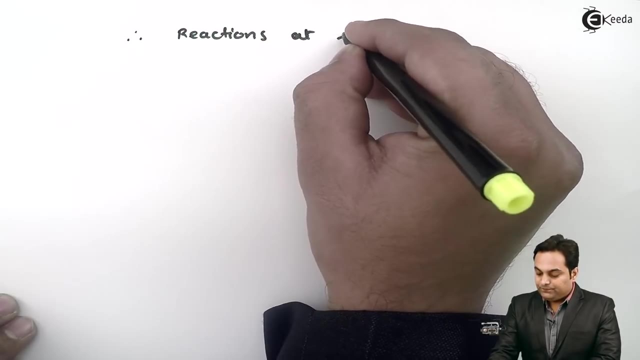 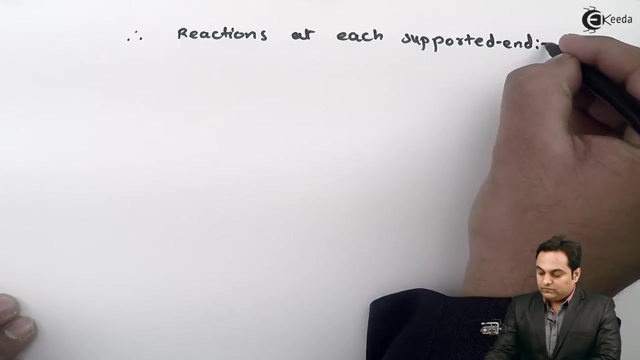 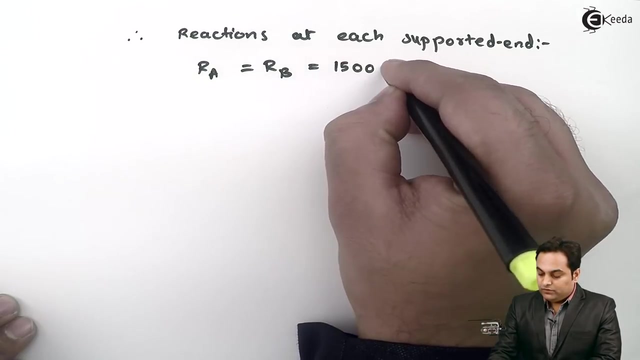 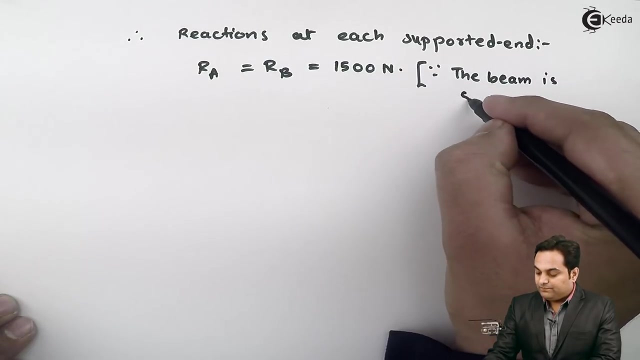 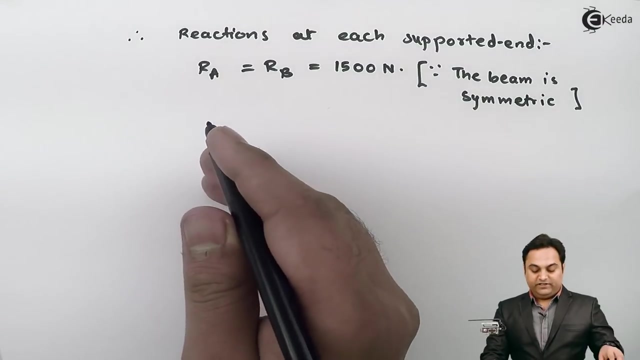 So next I will say that, therefore, reactions at each supported end, that would be R A, is equal to R B, and that is 1500 Newton. I can write down, since the beam is symmetric. Now, after getting this, I can say that therefore, 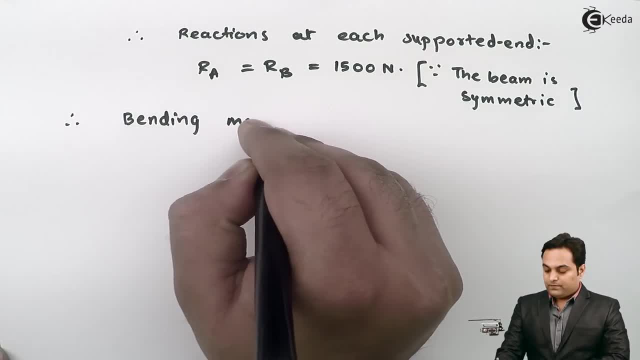 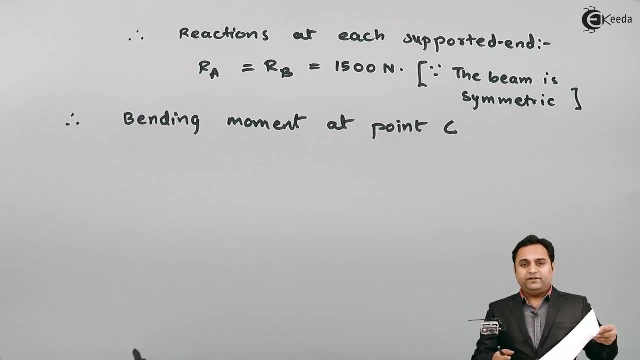 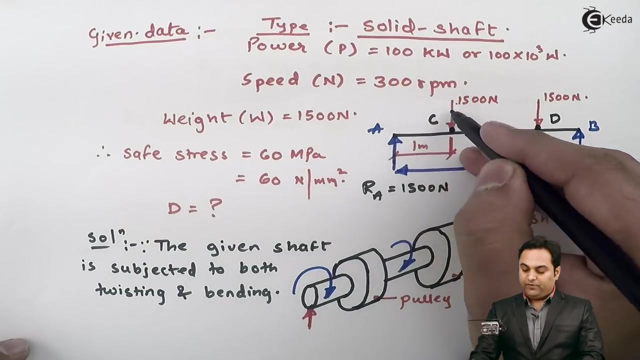 bending moment at point C. I can calculate either at point C or at point D. both the values would be same. So if I take the moment of this, 1500, it would be 1500 into 1. Because, as we know, moment is force into perpendicular distance. 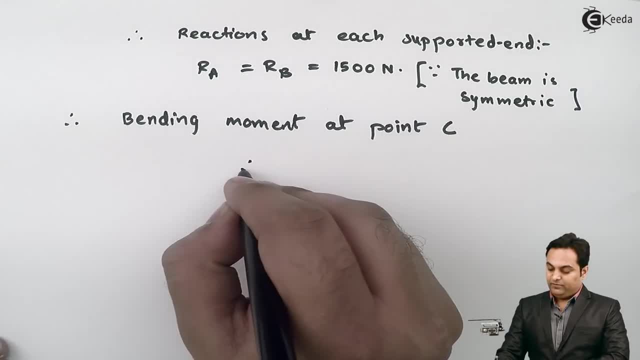 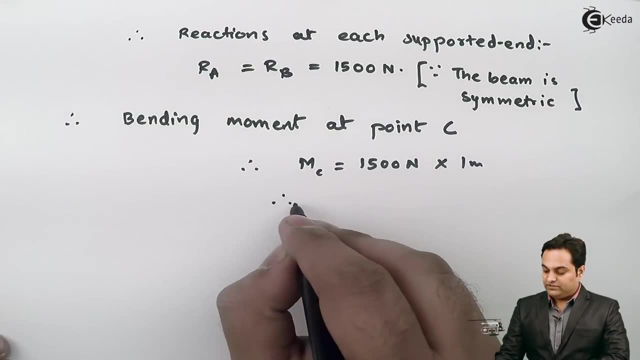 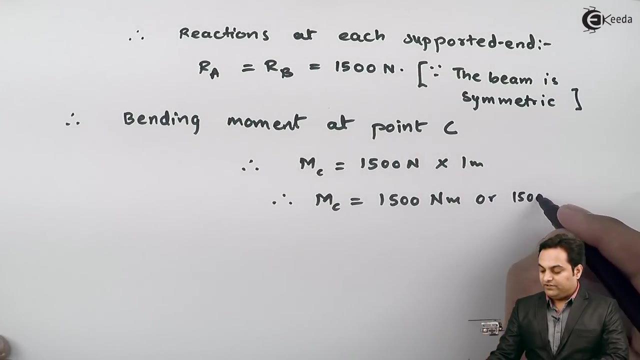 So it is 1500 into 1.. So therefore the bending moment at point C is equal to 1500 Newton into 1 meter. So hence moment at C is 1500 Newton meter, or I can write this as 1500 into 10 raised to 3 Newton millimeters. 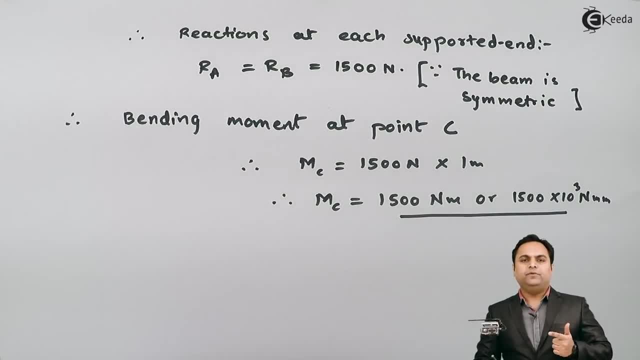 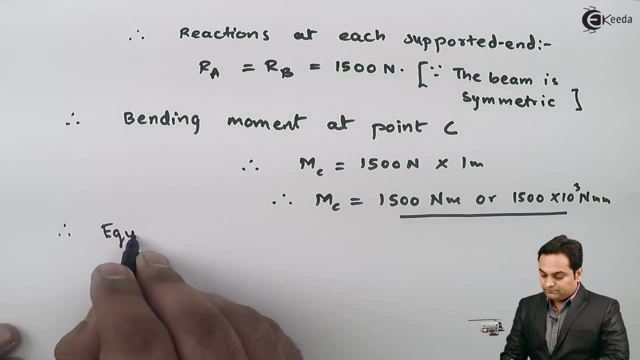 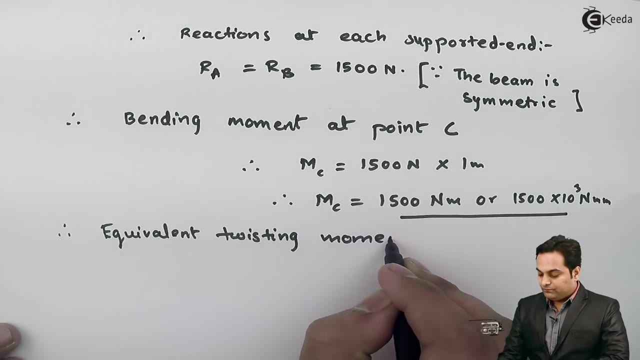 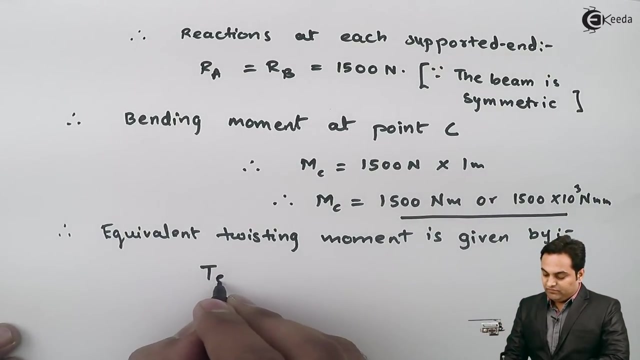 Now, once I know the value of twisting moment and bending moment, I can get the equivalent torque. I can say that, therefore, equivalent Twisting moment is given by the equivalent twisting moment is T equivalent, That is equal to square root of T square plus M square. 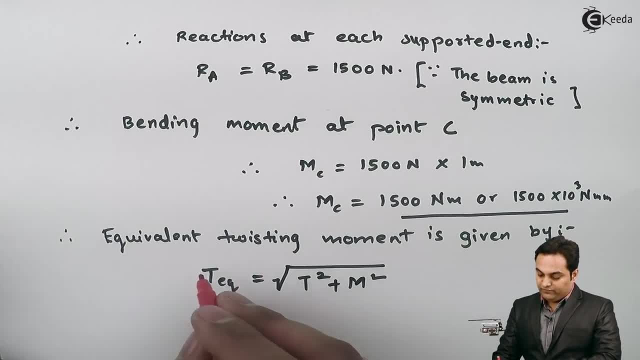 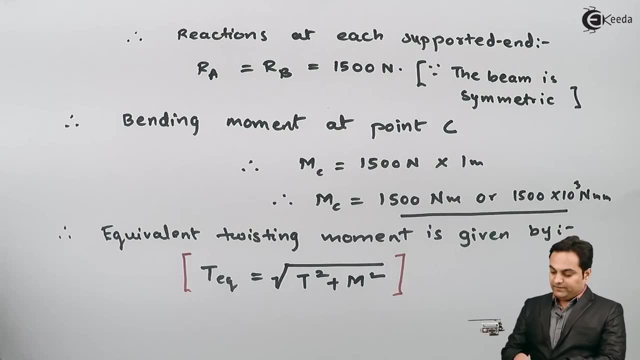 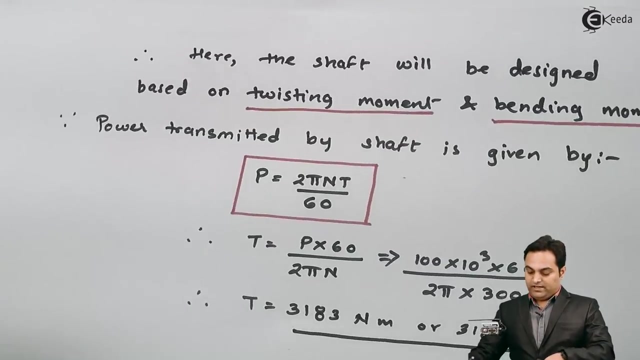 That is, it is the square root of torque and bending moment making square of that. So finally, I will say that, therefore, T equivalent will be equal to square root of the torque value which I am getting. That is, I have calculated it using the power and the torque was 3183 Newton meter. 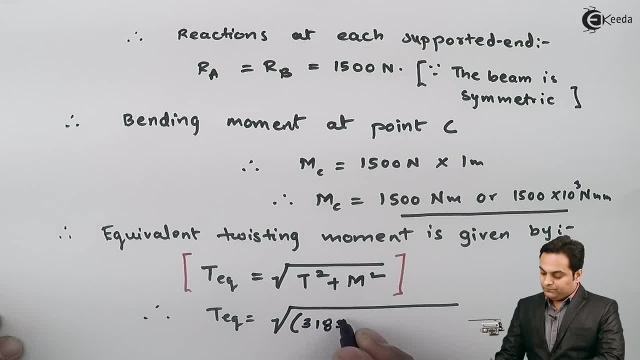 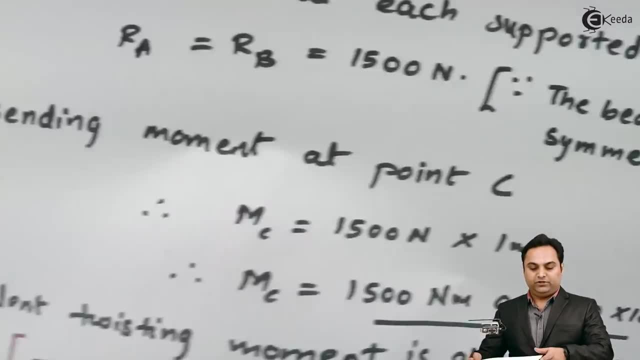 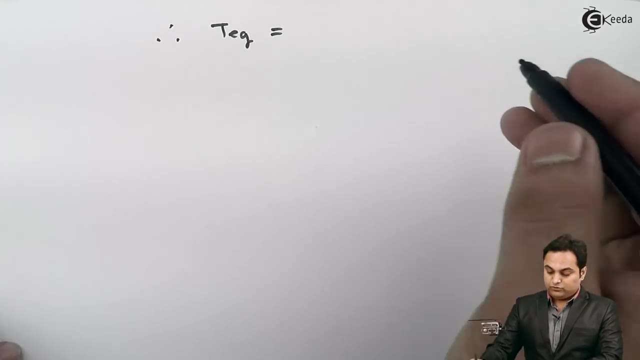 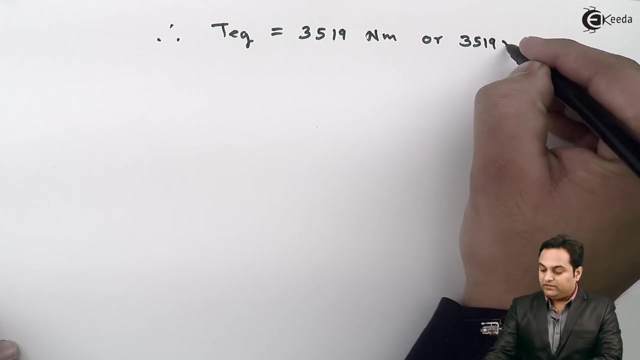 So it is 3183 plus bending moment is 1500.. So from this I will get equivalent torque And hence T equivalent. that comes out to be 3519 Newton meter, or it is 3519 into 10 raised to 3 Newton millimeters. 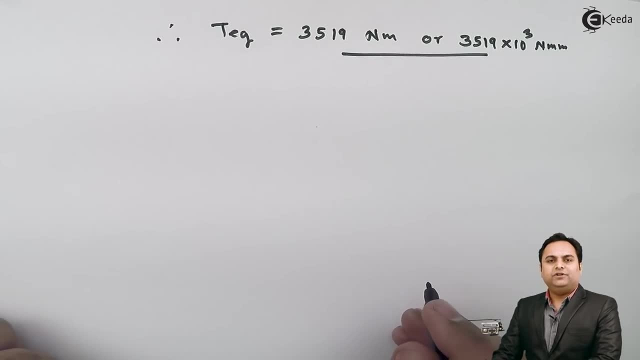 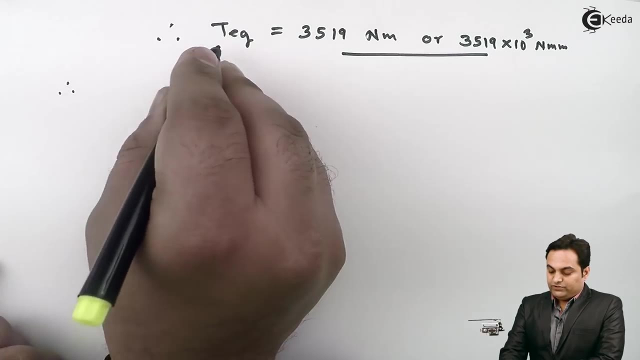 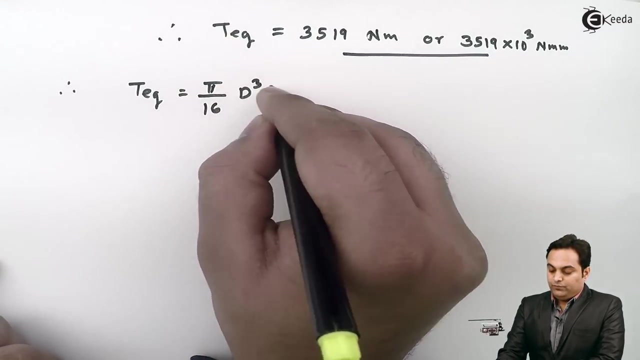 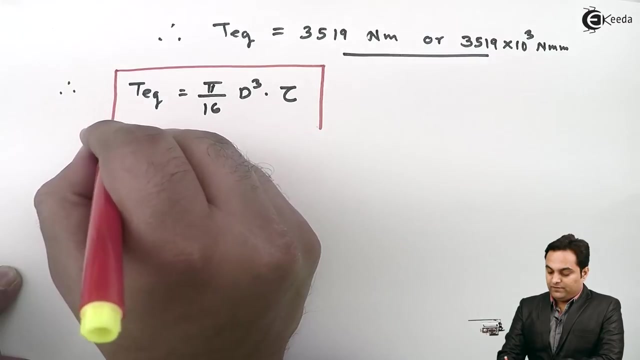 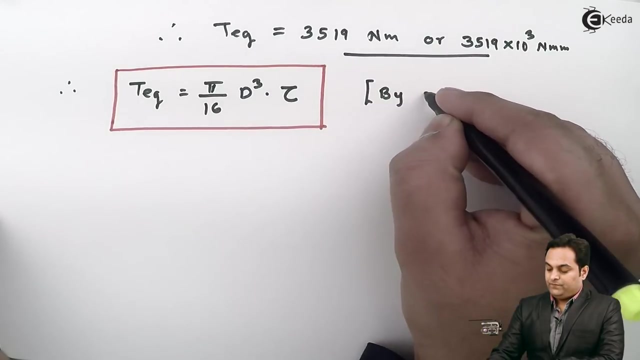 So, after getting equivalent torque now, I can easily calculate the diameter of shaft. I can say that, therefore, the equivalent twisting moment is also equal to that, is it? Therefore? we get the equivalent produce here, this, let us. 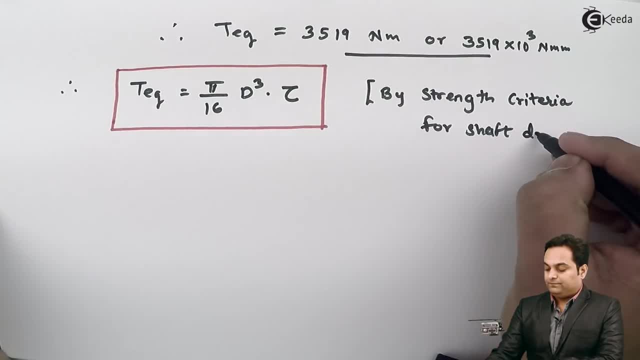 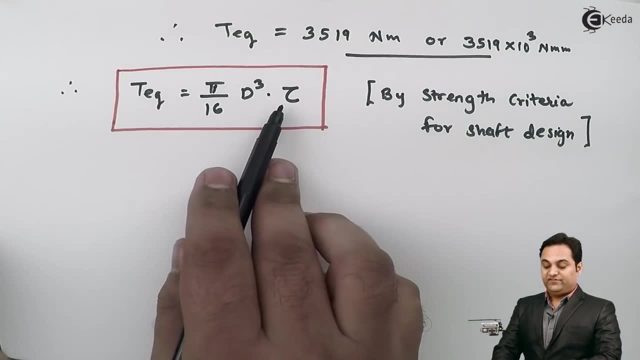 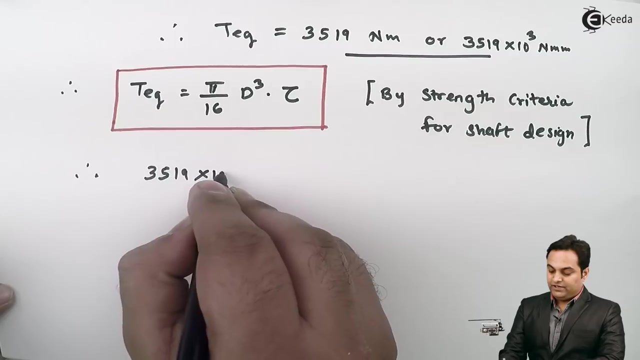 let us use this data here. this formula has come from the strength criteria. why? because here we have stress. so now I'll go on. putting the values: t equivalent is 3519 into 10, raise to 3. I'll put the value in Newton, mm, so that I get the answer of diameter in terms of. 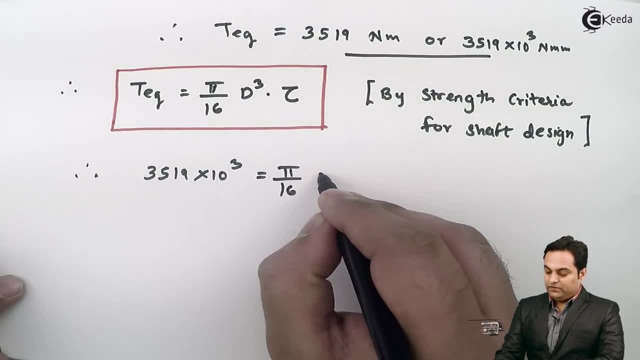 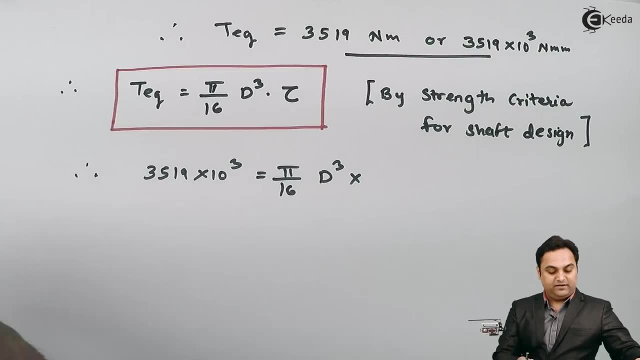 mm. it's equal to pi by 16 d cube. instead of tau. I can write the value- it is given the problem- as 60 mega Pascal. so it is into 60. so finally, d cube will be equal to 3519 into 10. raise to 3, this 16 will go on to one side, divided by pi into 60.